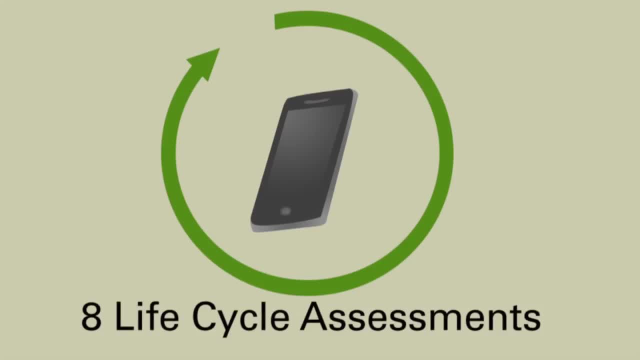 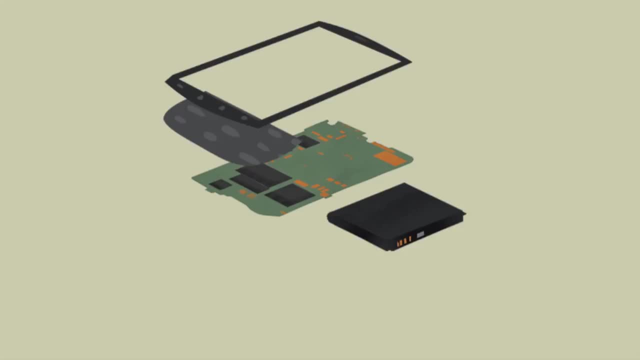 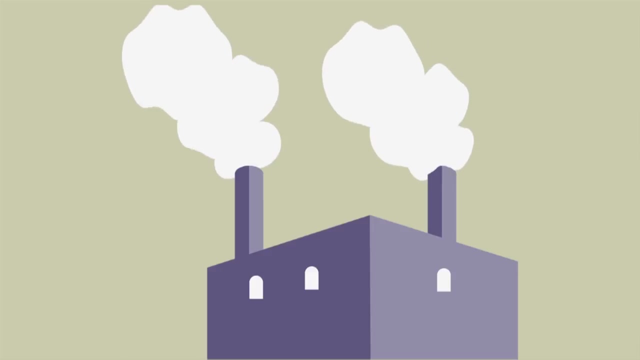 Mobile phones have eight life cycle assessments, one for each component. These include the printed circuit board, the display, the battery, the keypad, the microphone, the speaker, the plastic casing and any accessories. Now we are at the manufacturing stage of the life. 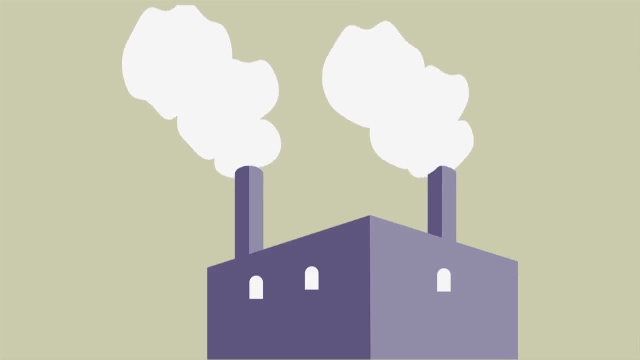 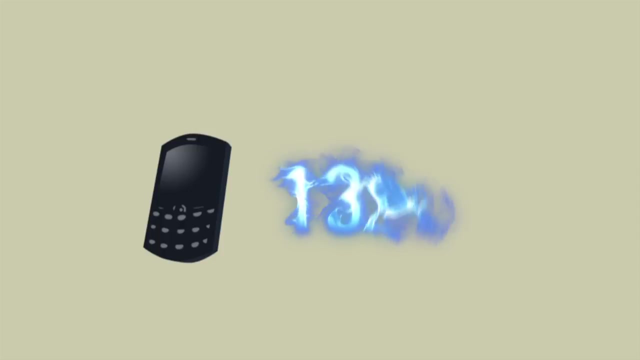 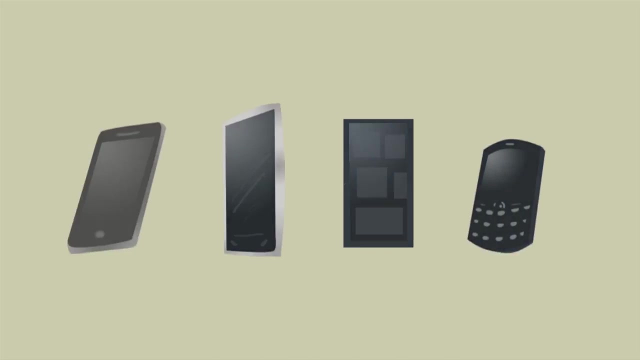 cycle assessment. Mobile phones made in factories require a great deal of energy to create. It is estimated that during manufacture, a single cell phone uses approximately 1390 millijoules of energy and produces 60 kilojoules of CO2 emissions. Many products require the 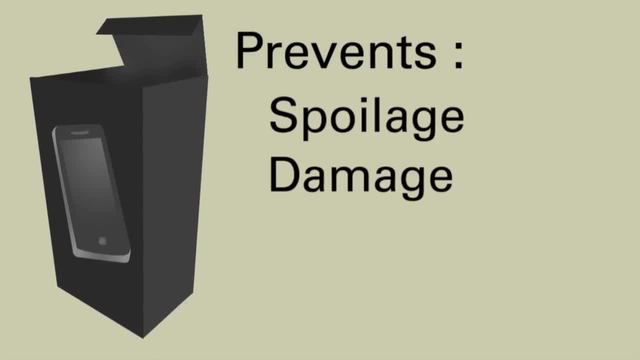 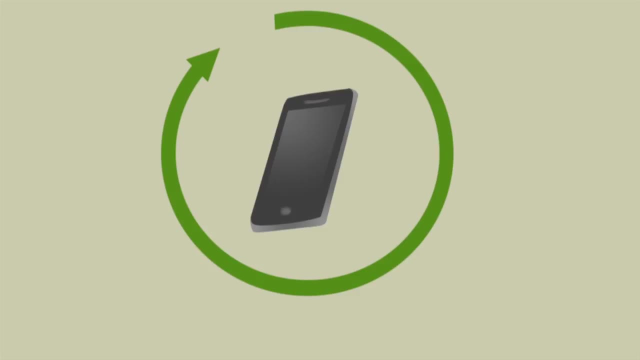 use of packaging as well, to prevent spoilage, damage, contamination and tampering. By considering the materials these phones are made of or reducing the number used in their manufacturing, this can lower some of the energy requirements. The next stage in the life cycle of a phone. 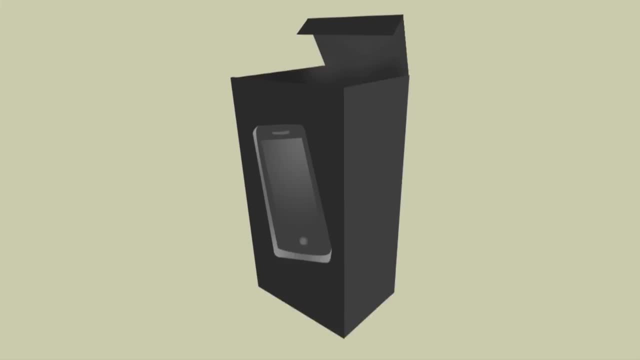 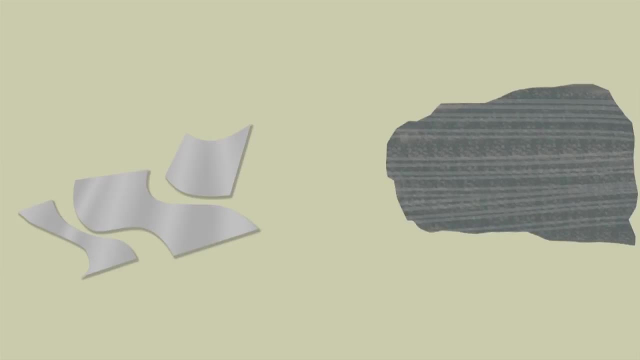 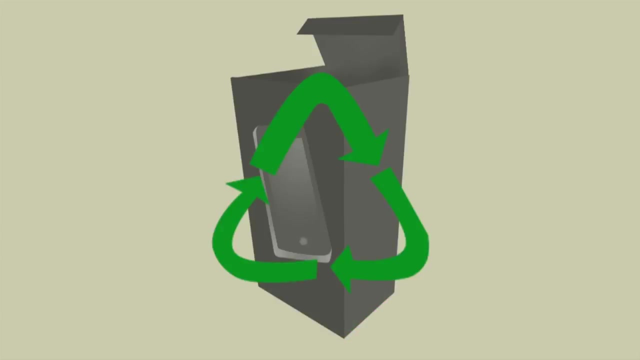 is its packaging and transportation. Packaging consumes valuable natural resources, such as paper from trees, plastic from crude oil in the earth, aluminium from ore or other materials, all of which use energy to extract and result in waste, Although some packaging can be made from recycled materials. in addition, the transport of a phone by plane, truck, radio. 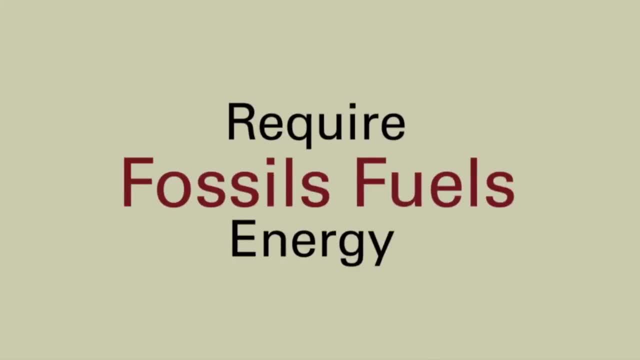 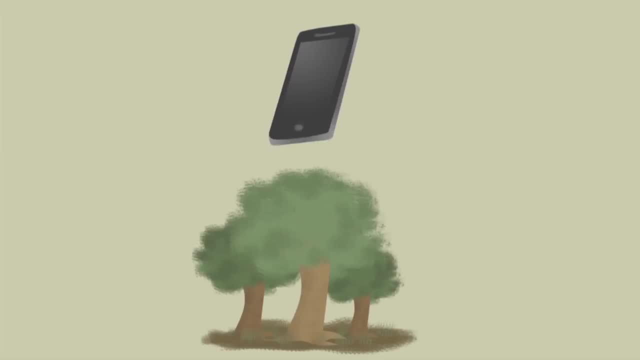 rail or sea all require use of fossil fuels for energy and contribute to global warming. Next, when making a mobile or cell phone, the environmental impacts during its useful life also have to be considered. The environmental impact of a phone is lower than, say, of a car. 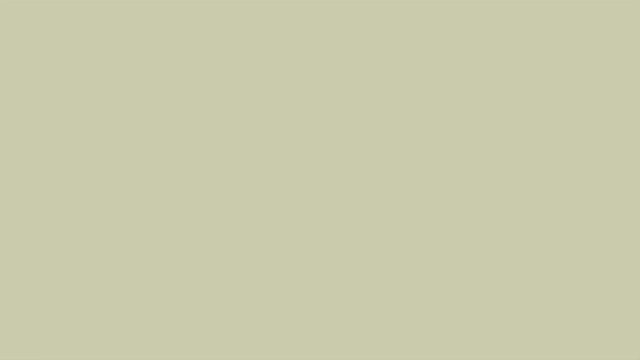 which burns fuel for its entire life. However, the lifetime of a mobile or cell phone is estimated that it is only between 18 to 24 months. This means that existing phones are exchanged for newer models, So more and more old phones are being dumped. One way to extend. 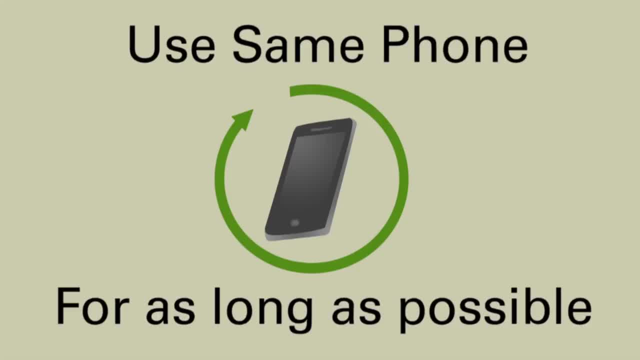 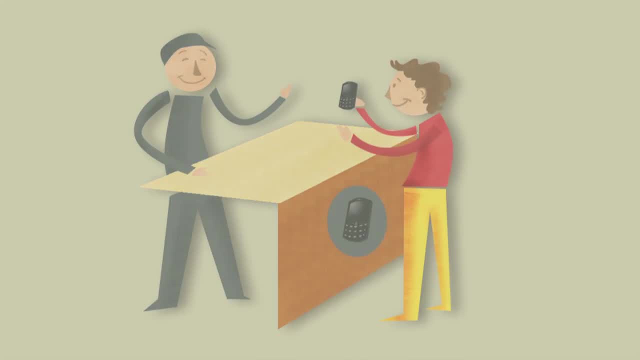 the useful life of your phone and prevent waste is to use the same phone for as long as possible. When you shop, try to make sure you get the service and the phone that's right for you. Inevitably, each phone will come to the end of its useful life. This is the